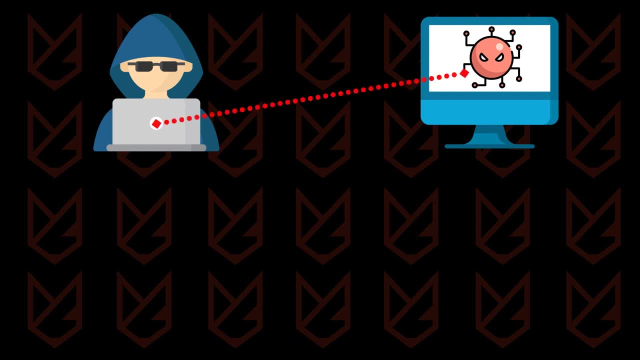 has a Trojan. the hackers could access your PC anytime. They can access your files, make changes to them, steal your confidential files. It is also used to spy on other people. For example, hackers might get your banking information and can steal your money Also. they can use 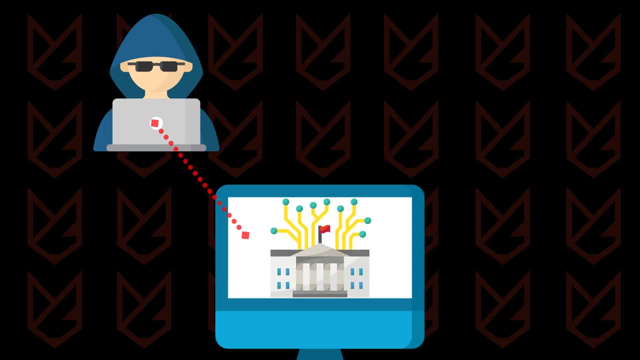 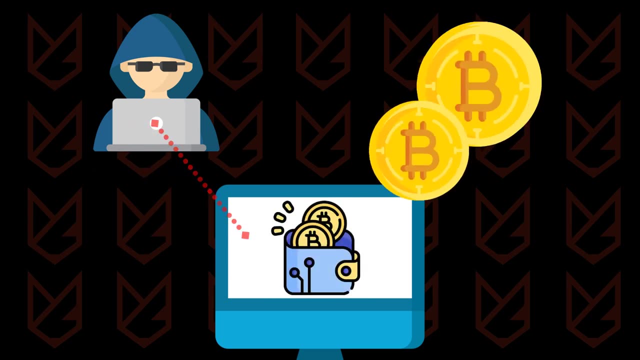 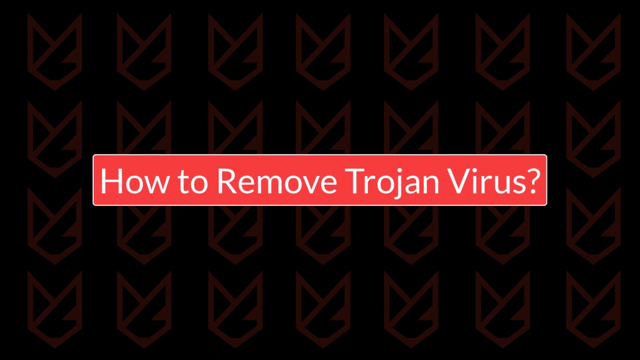 your computer to do other illicit activities, such as hacking secure government networks so that the officer arrests you. instead of them, They can also use your computer to harvest cryptocurrencies, which will drastically impact your system performance. How to remove a Trojan virus. Now that you know your PC has a Trojan infection, you should perform the removal steps in the 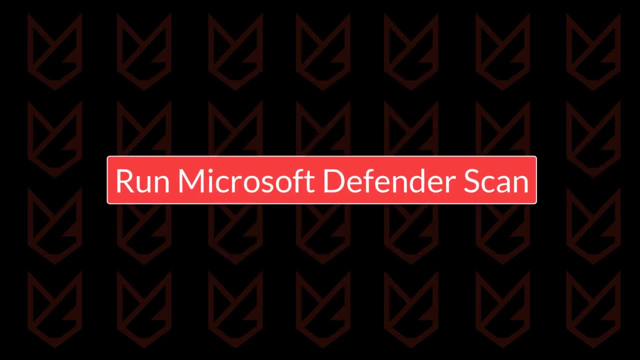 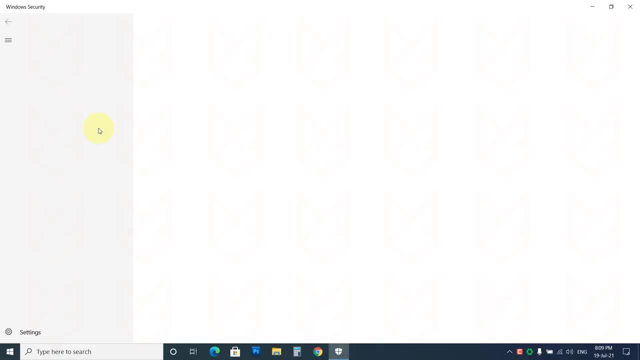 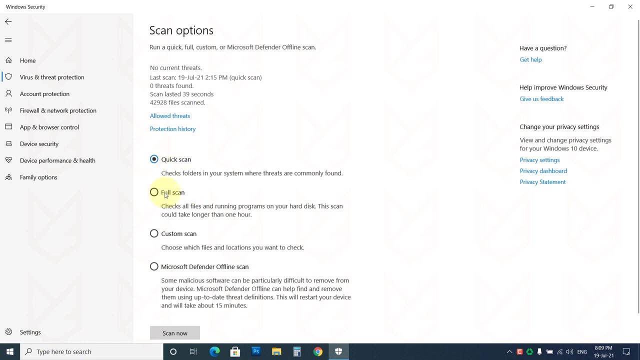 correct order to clean your computer: Run Microsoft Defender Scan. Click on your Start menu and type Windows Security. Open it Now. click on Virus and Threat Protection. Now click on Scan Options. Select Full Scan, then click on Scan Options. Now click on Scan Options. 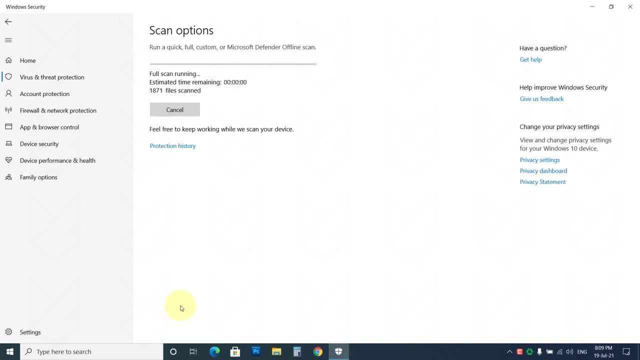 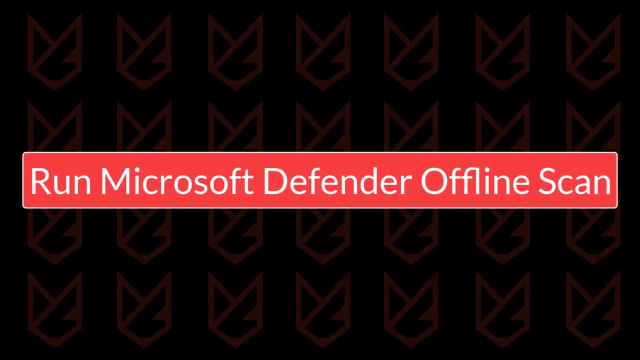 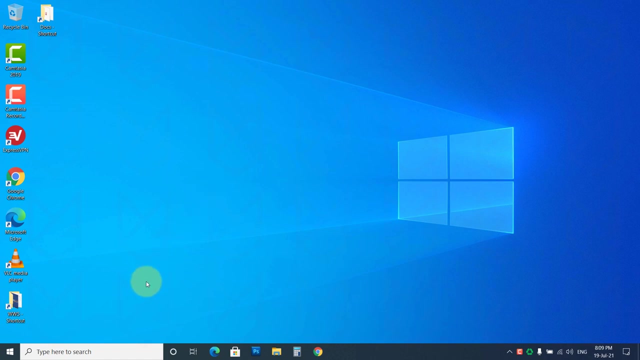 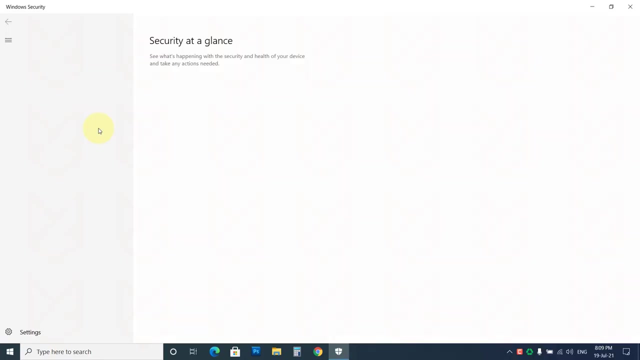 Now wait for the scan to complete. Then remove all the detected threats. To scan your Froge and Red. Whenever you control your touch screen, click on CAN Run Microsoft Defender Offline Scan. Some trojans are difficult to remove and they hide in your PC pretending to be a system file, So you should run the Defender Offline scan to catch such threats. 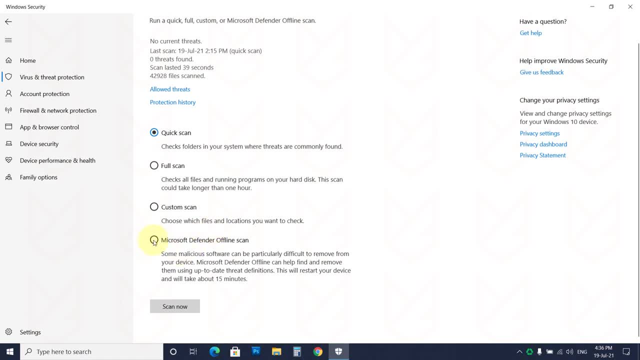 Click on your Start menu and type windows security- Open it Now click on Virus and Threat Protection. Now click on Scan Options. Select the Microsoft Defender Offline Scan, then click on Scan Now. Now your PC will restart and the scan will take place offline. 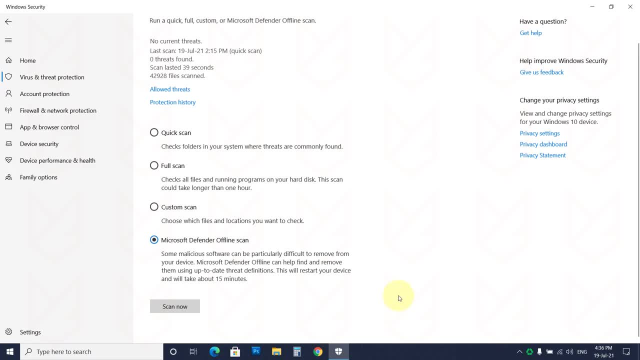 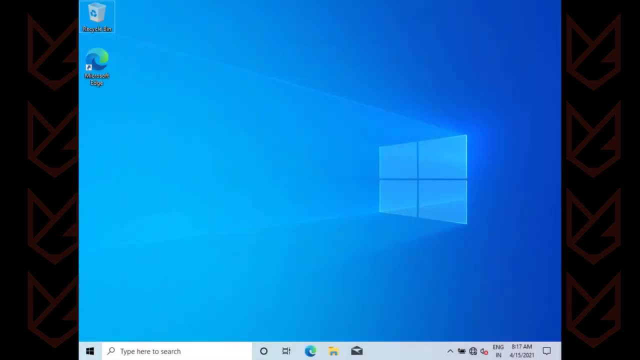 Now follow the next fixes to remove the Trojans completely. Boot in Safe Mode. If you boot the Windows 10 in Safe Mode, malware removal becomes easy. In Safe Mode, only essential services and processes run, so you can easily clean your PC. 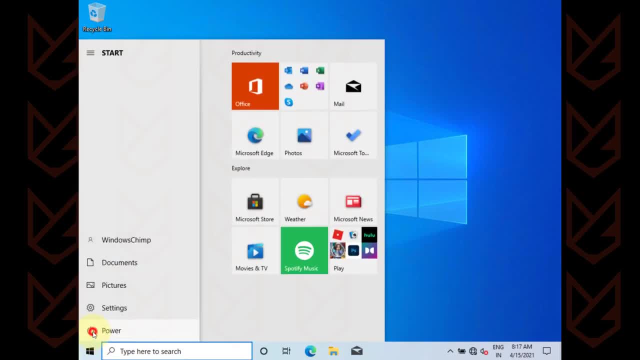 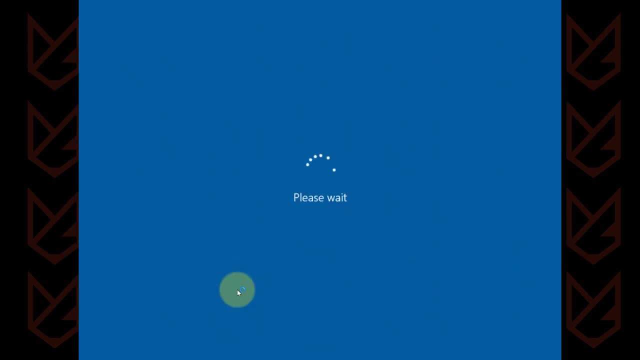 To boot in Safe Mode. click on the Start menu. Go to the Power Options. Now press the Shift button and click on Restart. After that your system will go to Full Screen Mode. Now go to the Troubleshooting, then Advanced Options. 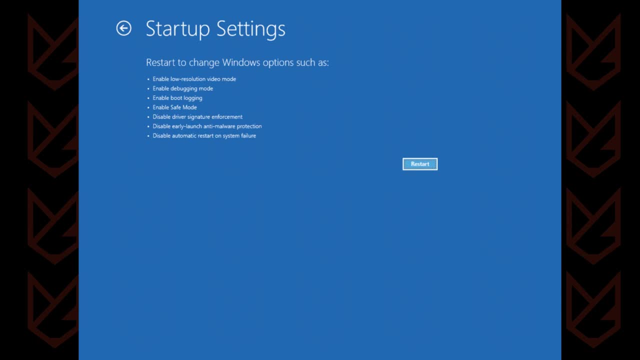 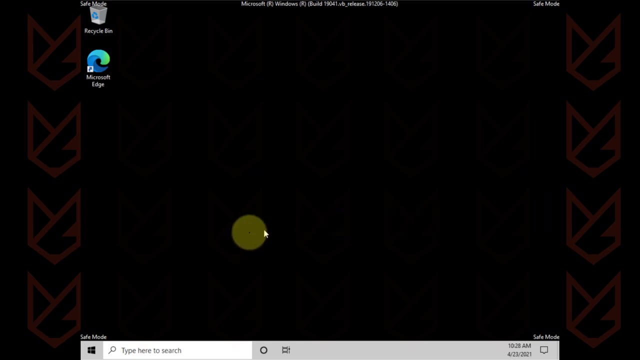 Now click on Startup Settings, then Restart button. Your system will boot in the Safe Mode. You can now perform the next steps to clean the malware. Delete temporary files. Most malware hides in the temporary files. They load as temporary files and then start infecting your system. 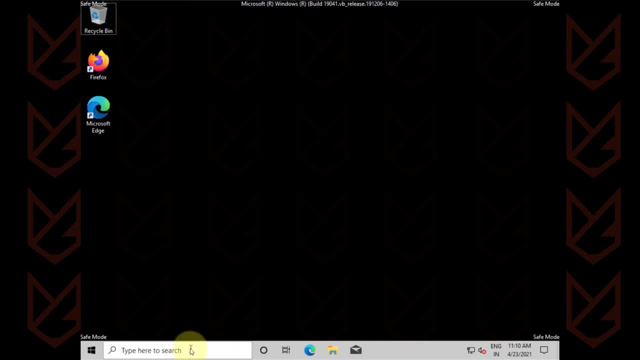 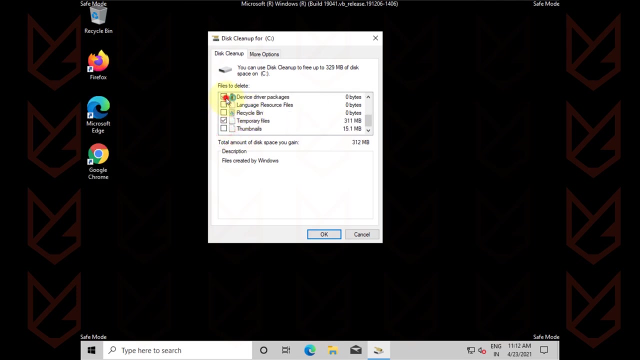 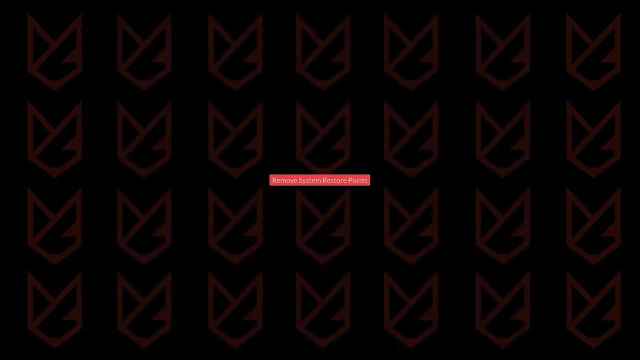 So your first step should be deleting the temporary files. To do that, click on the Start menu and type Disk Cleanup. Click on it to open. Click OK. Now deselect everything and select Temporary Internet Files and Temporary Files. Click OK. Then confirm your action by clicking on Delete Files. 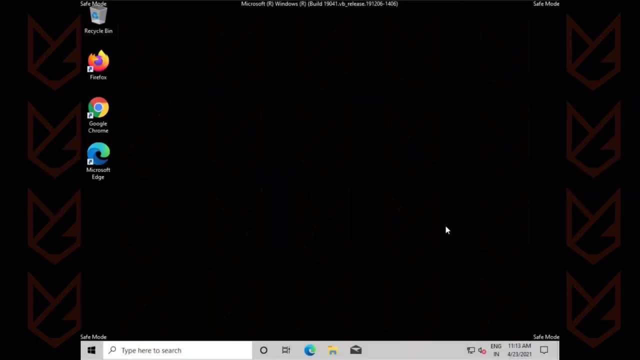 Remove system restore points. System restore points are used to restore the system to a working state. If any problem happens with the computer, the user tries to restore it to a restore point. Malware creators are aware of this, so they create the malware to infect the system restore points also. 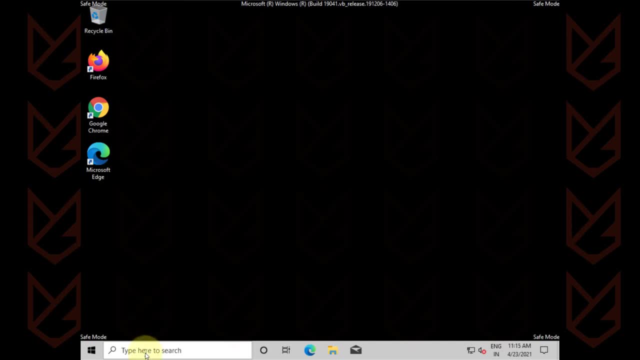 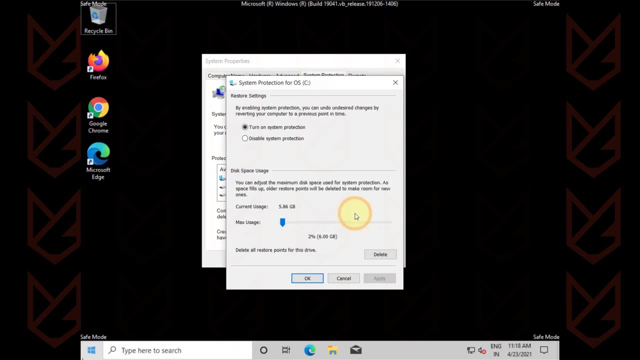 It is better to remove the system restore points. Click on the Start menu And type Create a restore point. Open it, Then click on Configure. Click on Disable system protection, Then click on the Delete button to delete all the system restore points. 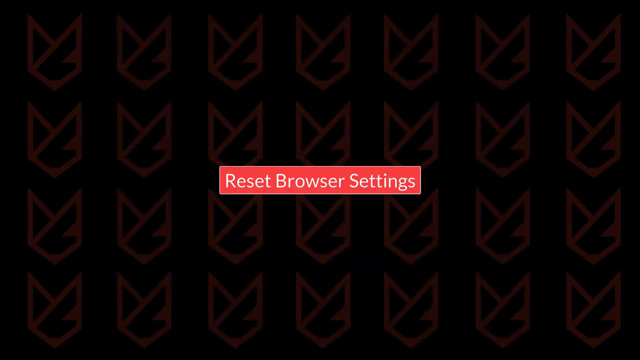 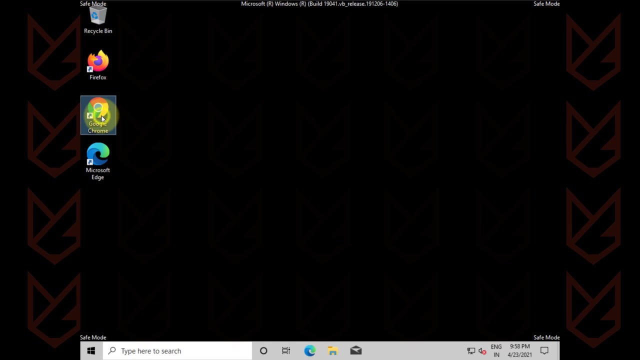 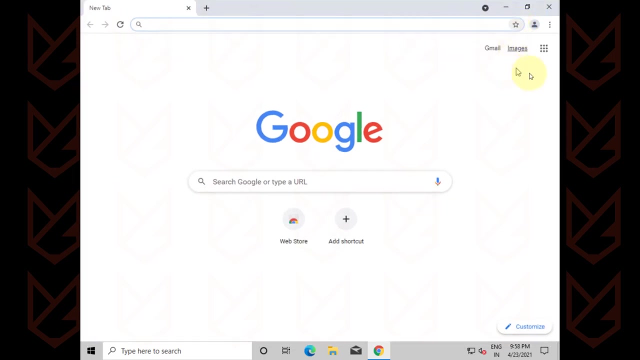 Click on Continue to confirm. Reset browser settings. Malware hijacks the settings of your browser and redirects you to malicious sites so that they can infect your system with malware again. You should reset the browser's settings to avoid that. To reset the settings of Google Chrome, click on the Menu button. 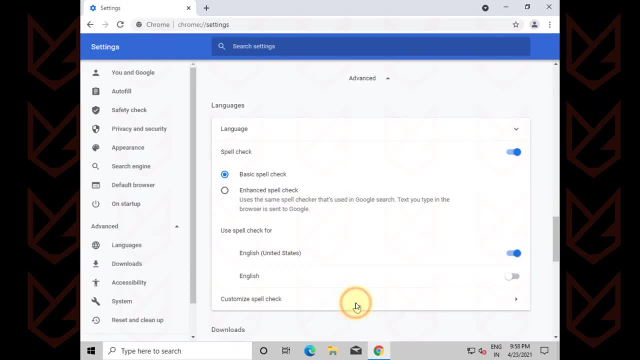 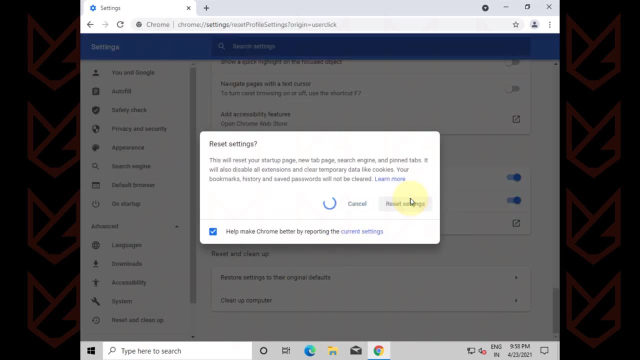 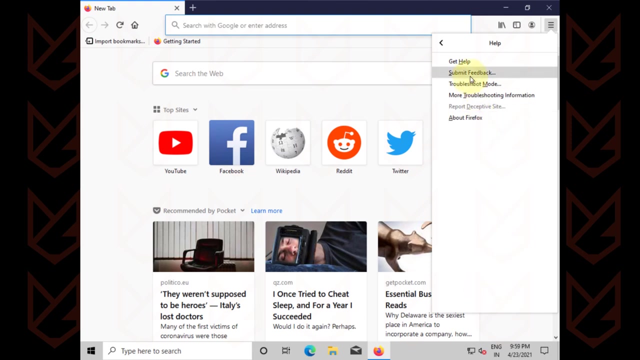 Then Settings, Advanced. Then click on Restore settings to their original defaults. Now confirm your action. To reset the settings of Mozilla Firefox, click on the Menu button, Then Help, Then click on Troubleshooting information. Now click on Restore. Now click on Refresh Firefox. 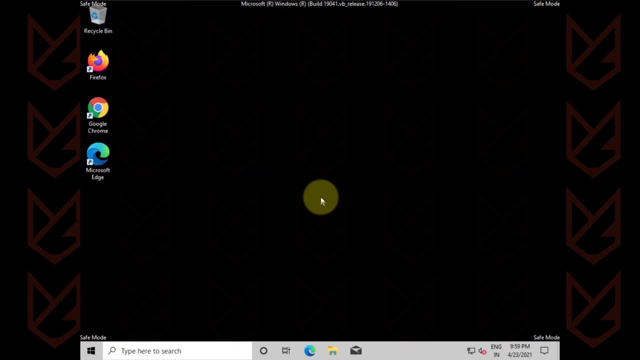 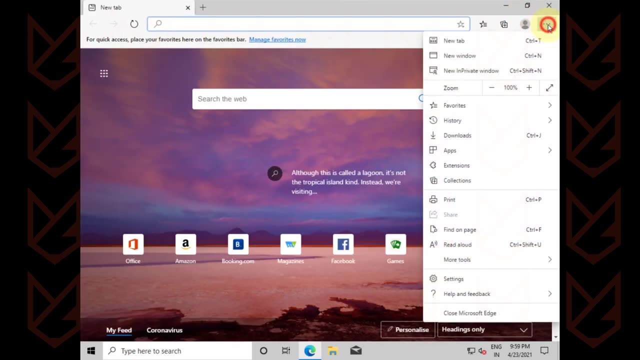 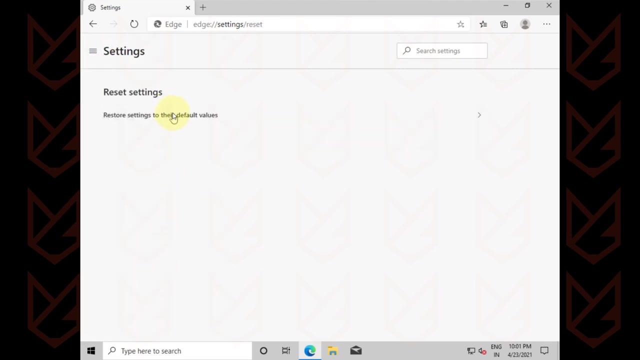 Now click on Refresh Firefox again to confirm your action. If you are using Microsoft Edge, open the Menu. Then go to Settings. Click on Reset settings from the left sidebar. Now click on Restore settings to their default values. Then confirm your action by clicking on the Reset button.